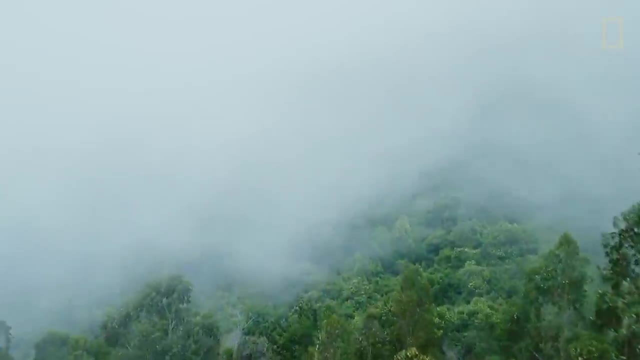 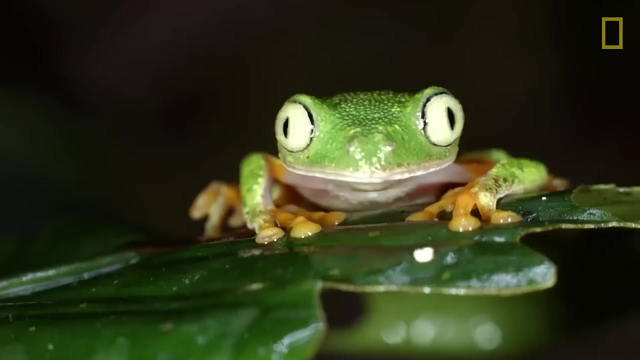 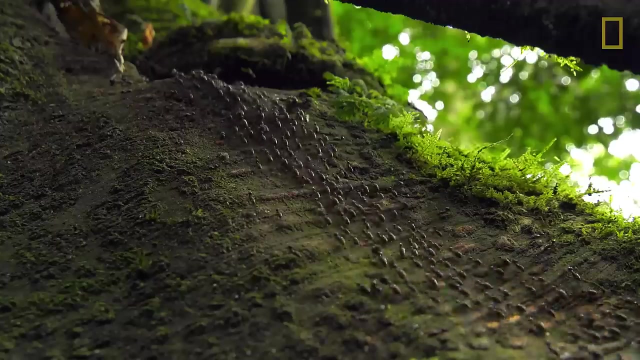 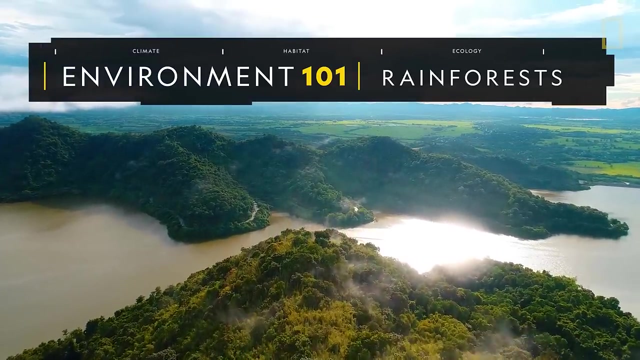 Shrouded in a blanket of clouds, they awaken. Their canopies of green glitter in the sun. Their wildlife start to slither, chirp and growl And one of the planet's richest ecosystems comes to life. Rainforests are the oldest living ecosystems on the planet. Some can trace their origins to over 70 million years ago, back to a time when dinosaurs still roamed the earth. While the giant reptiles have disappeared, rainforests continue to thrive, growing on every continent except Antarctica. Two types of rainforests are scattered across the globe: temperate and tropical Temperate. 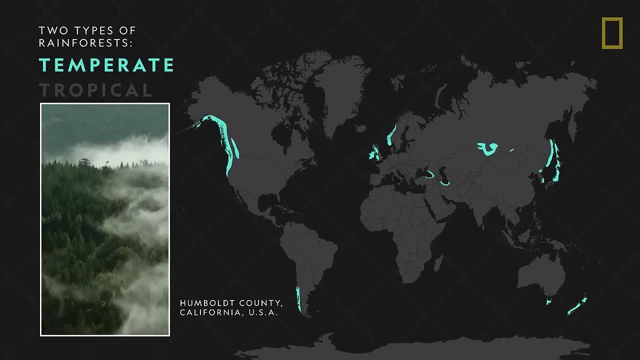 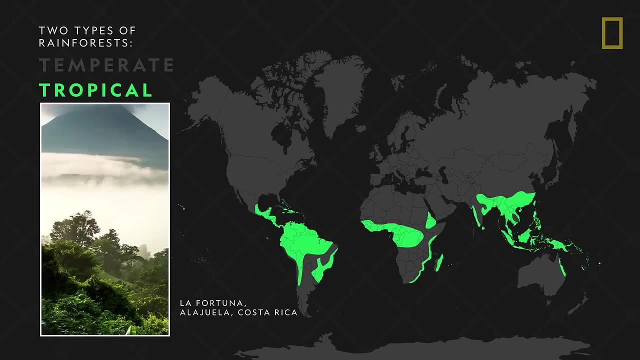 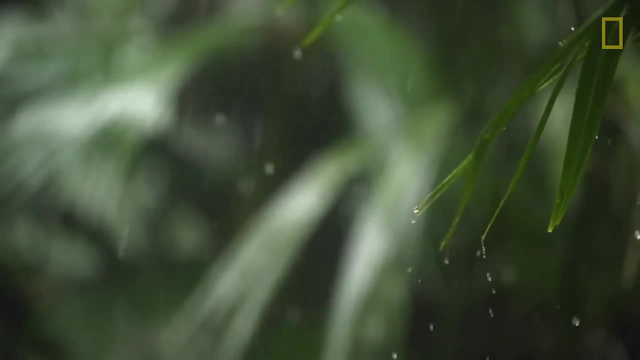 rainforests are mainly found in the mid-latitudes, often near cooler coastal mountainous regions. Tropical rainforests are primarily located in warmer climates between the Tropic of Cancer and the Tropic of Capricorn. As their names imply, temperate and tropical rainforests. 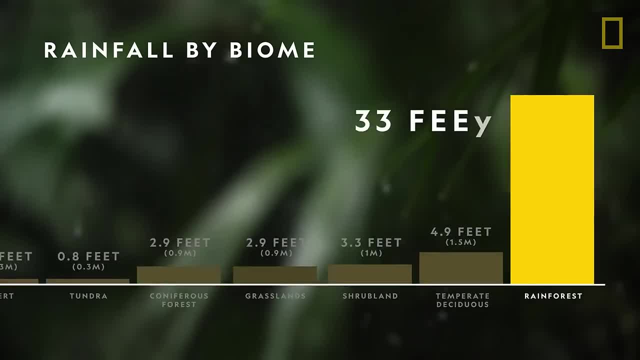 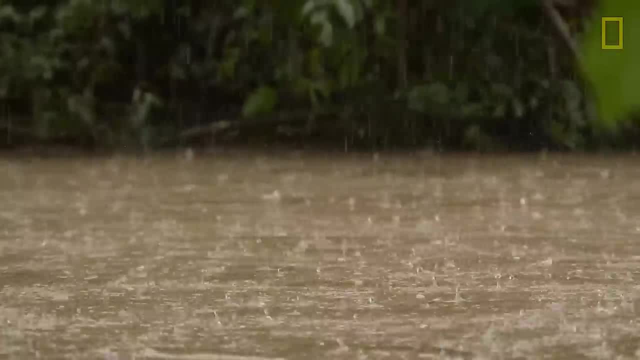 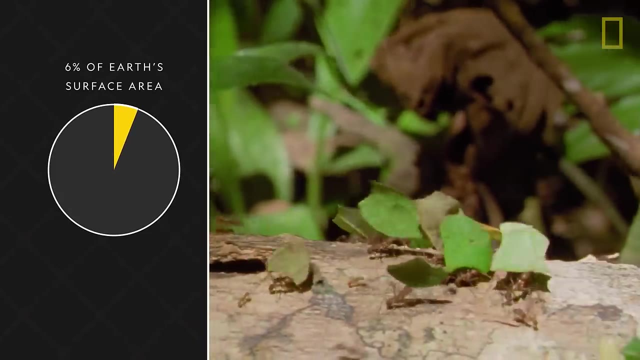 are the wetlands of tropical rainforests. The rainforests are the most wet forest on Earth, receiving up to about 33 feet of rain per year. This precipitation plays a critical role in creating an exceptionally lush and biologically diverse habitat. While rainforests only make up about 6% of the Earth's surface area, they 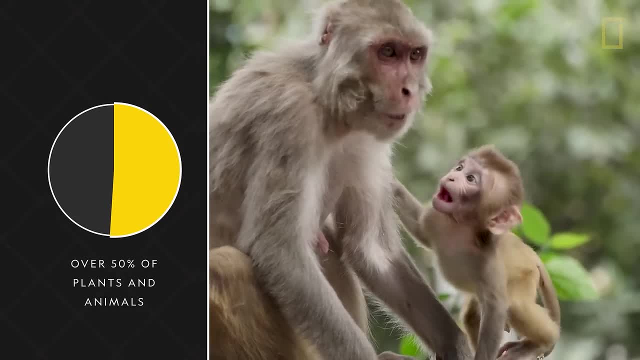 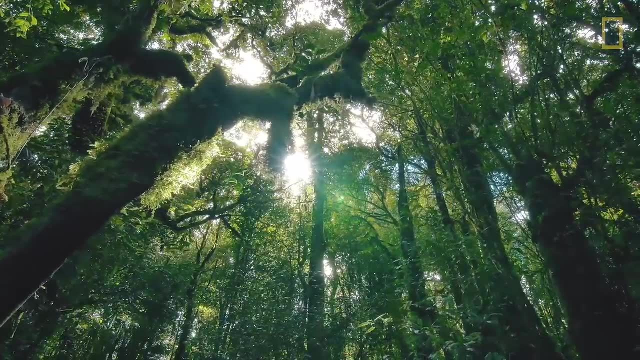 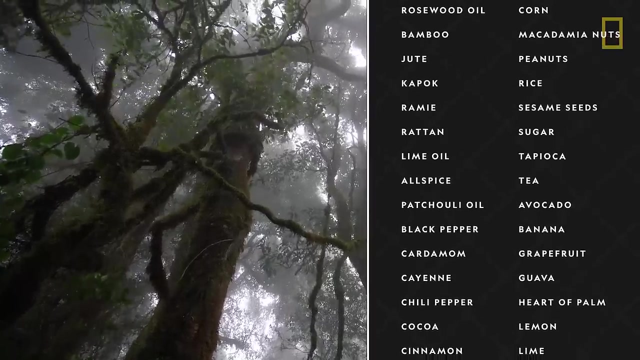 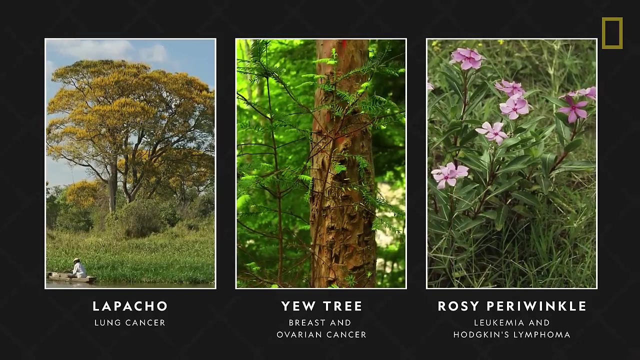 are home to over half of the world's plant and animal species. This biodiversity creates benefits that extend far beyond the reach of the earth's surface. The rainforest plants produce an assortment of food items, in addition to ingredients useful in everyday products and medicines. In fact, an estimated 70% of the plants used 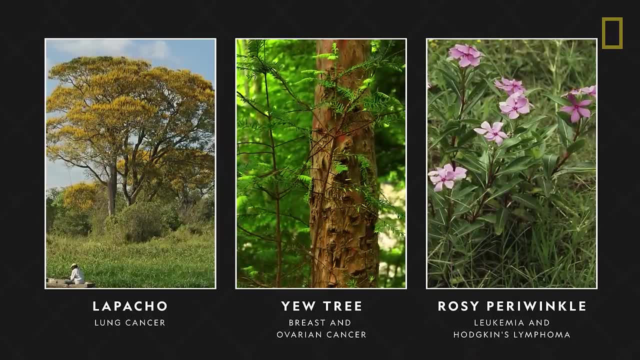 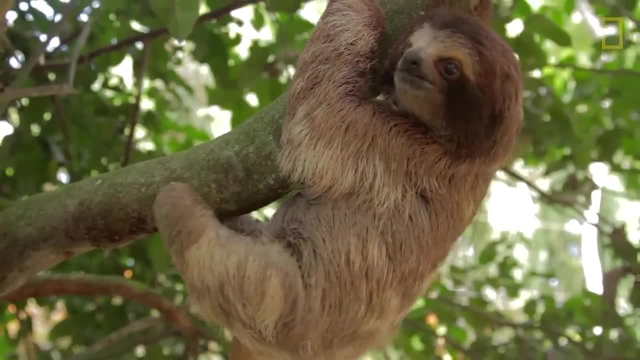 in cancer, treatments are only found in rainforests. On an even larger scale, rainforests help to stabilize the planet's climate. Its lush green vegetation regulate global temperature and its natural habitat On an even larger scale. rainforests help to stabilize the planet's climate. Its lush green vegetation regulate global 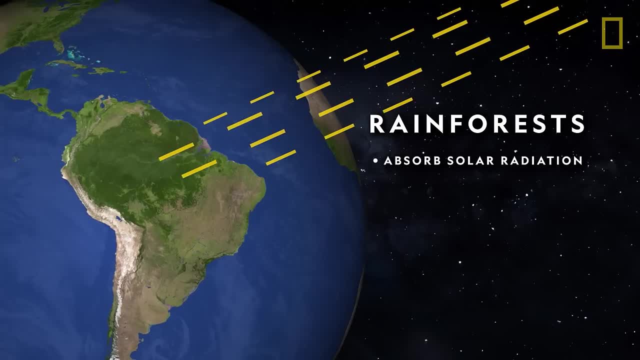 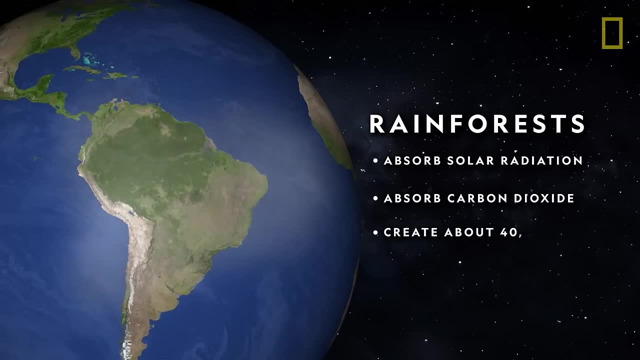 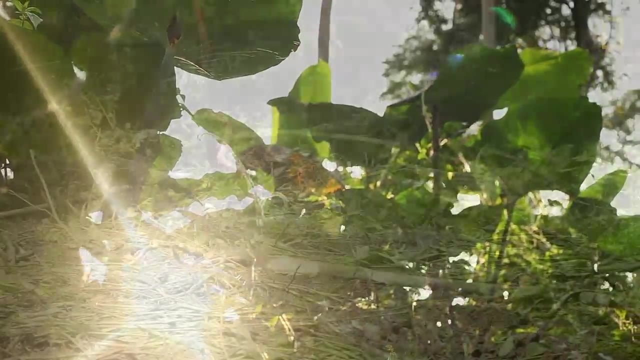 temperatures. by absorbing massive amounts of radiation from the sun, They also absorb vast amounts of carbon dioxide and convert them into oxygen- about 40% of the planet's breathable air. Over the past few centuries, rainforests have disappeared at an alarming rate. Factors such as economic inequalities, human development and demand for natural resources have fueled the deforestation of these rich ecosystems. At the current rate, rainforests which have survived for over 70 million years may completely disappear within the next century. 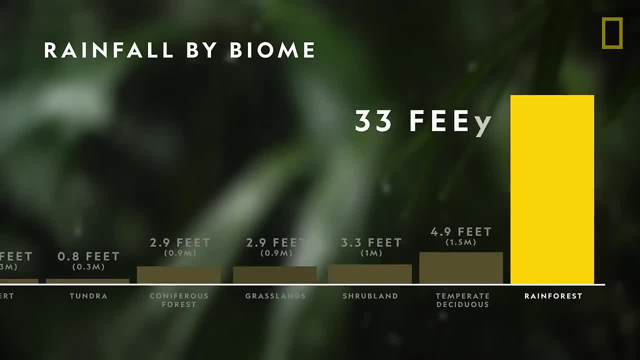 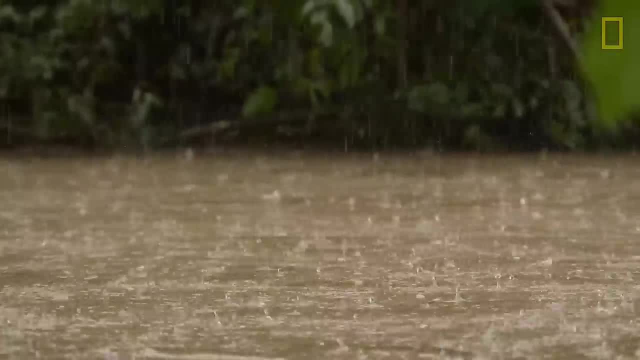 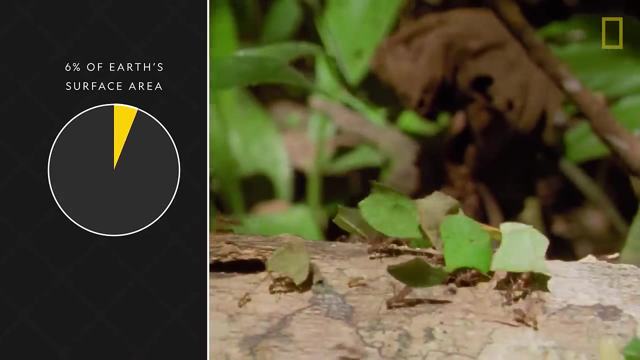 are the wetlands of tropical rainforests. They are the wettest forests on earth, receiving up to about 33 feet of rain per year. This precipitation plays a critical role in creating an exceptionally lush and biologically diverse habitat, While rainforests only make up about 6% of the earth's surface area. 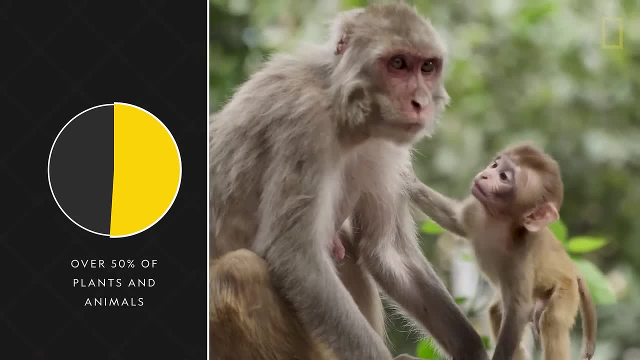 they are home to over half of the world's plant and animal species. This biodiversity creates benefits that extend far beyond the reach of the earth's surface. This biodiversity creates benefits that extend far beyond the reach of the earth's surface. This biodiversity creates benefits that extend far beyond the reach of the earth's surface. 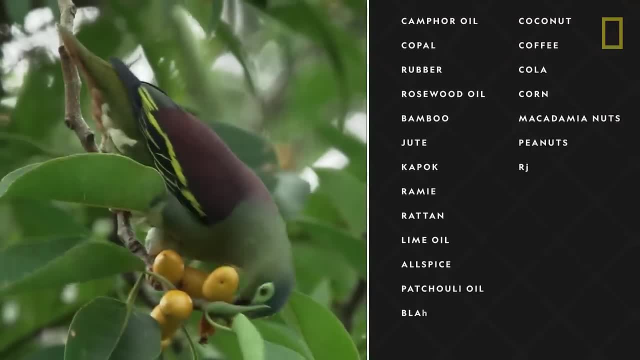 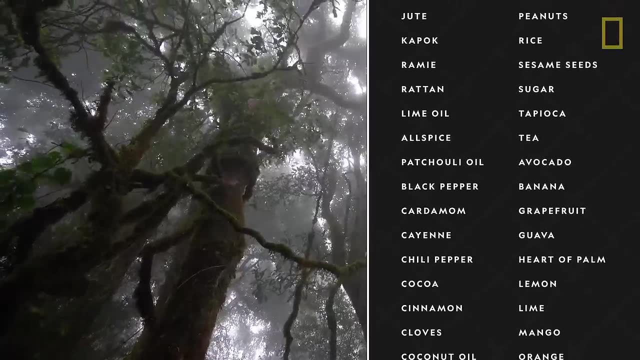 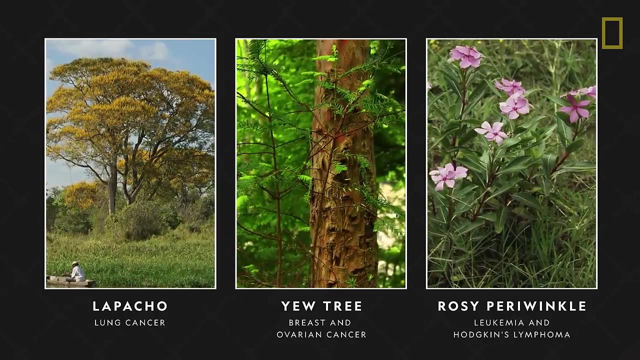 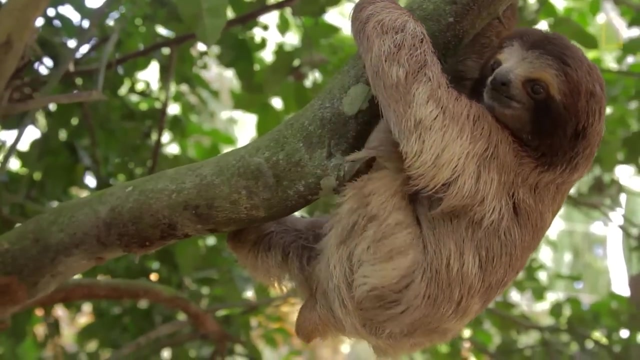 Rainforest plants produce an assortment of food items, in addition to ingredients useful in everyday products and medicines. In fact, an estimated 70% of the plants used in cancer treatments are only found in rainforests. On an even larger scale, rainforests help to stabilize the planet's climate. Its lush. 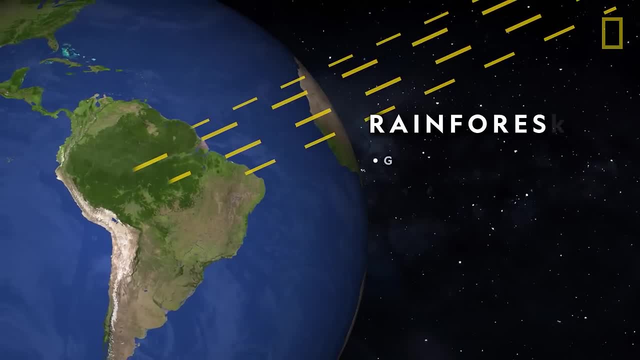 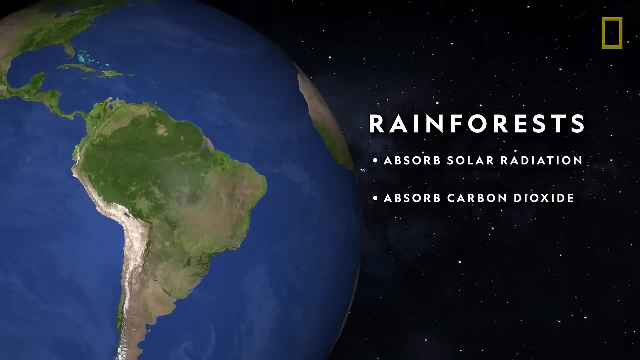 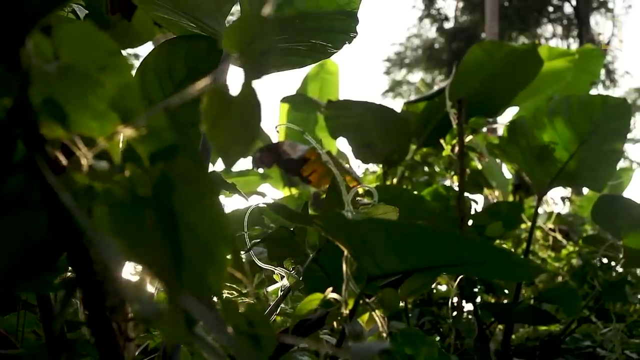 green vegetation regulate global temperature and climate control. Rainforest plants are able to control global temperatures by absorbing massive amounts of radiation from the sun. They also absorb vast amounts of carbon dioxide and convert them into oxygen- about 40% of the planet's breathable air. 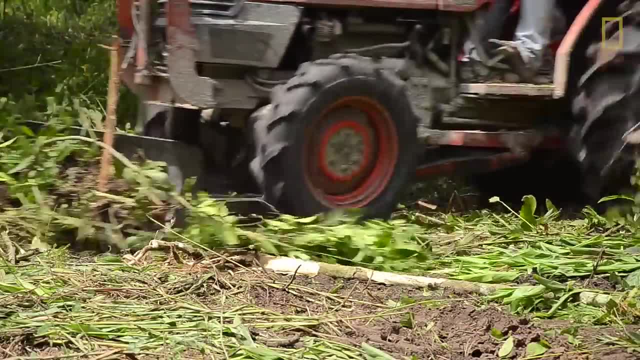 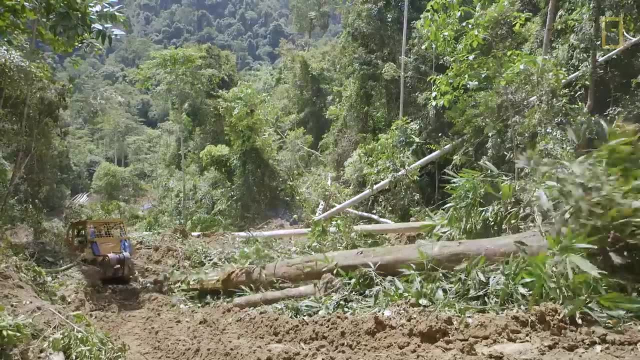 Over the past few centuries, rainforests have disappeared at an alarming rate. Factors such as economic inequalities, human development and demand for natural resources have fueled the growth of rainforests. In the past few centuries, rainforests have disappeared at 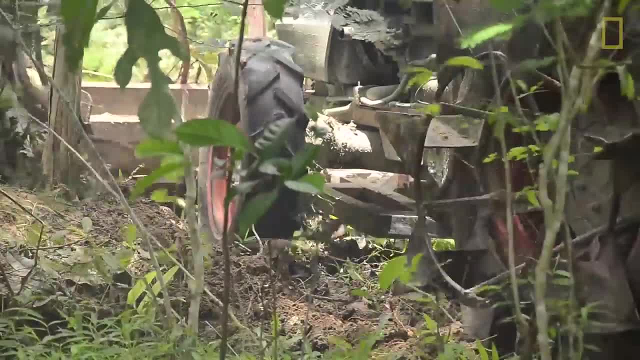 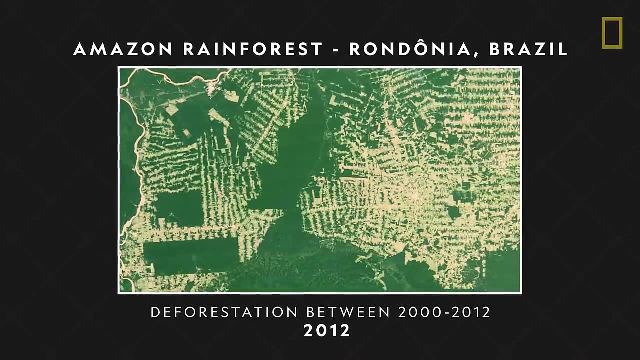 an alarming rate. Factors such as economic inequalities, human development and demand for natural resources have fueled the growth of rainforests. Deforestation has been the largest cause of deforestation in the world. At the current rate, rainforests which have survived for over 70 million years may completely 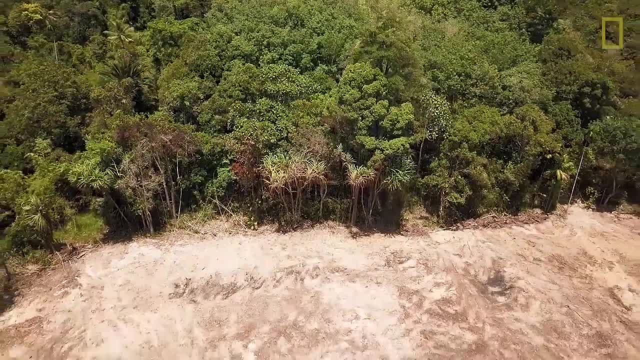 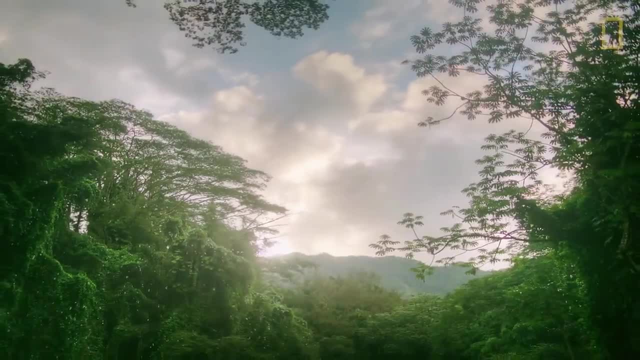 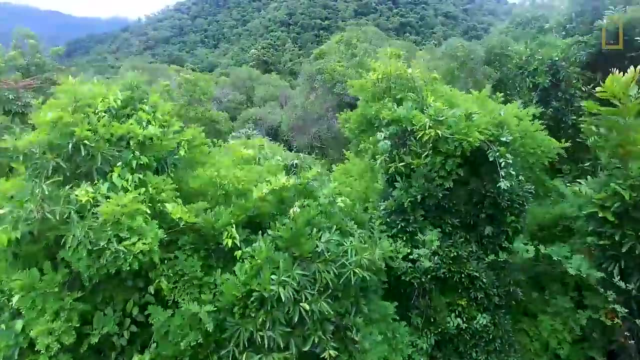 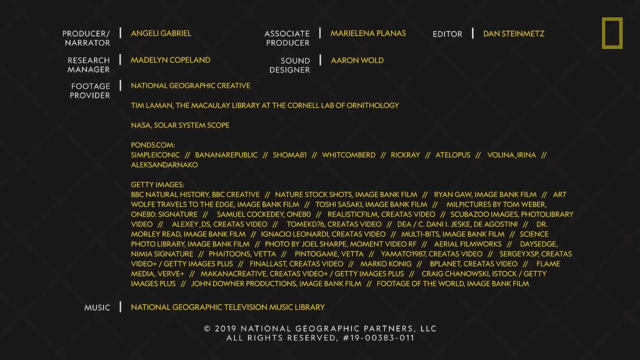 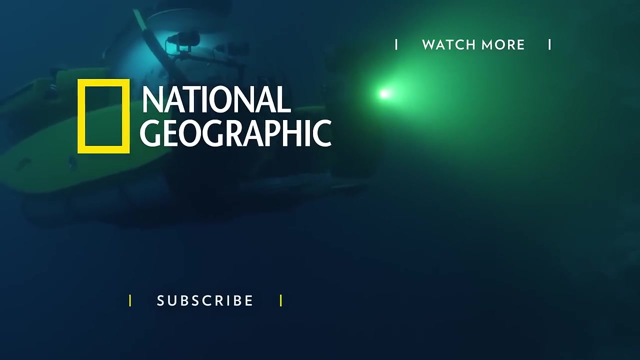 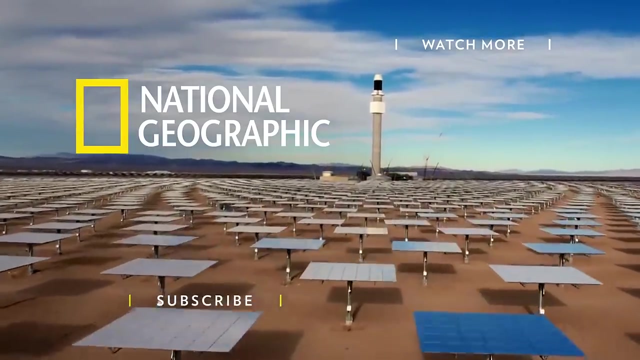 disappear within the next century. But through educational campaigns, sustainable logging practices and cooperation with local communities, deforestation may begin to slow down, helping preserve rainforests for many generations to come. Transcription by ESO. Translation by —.